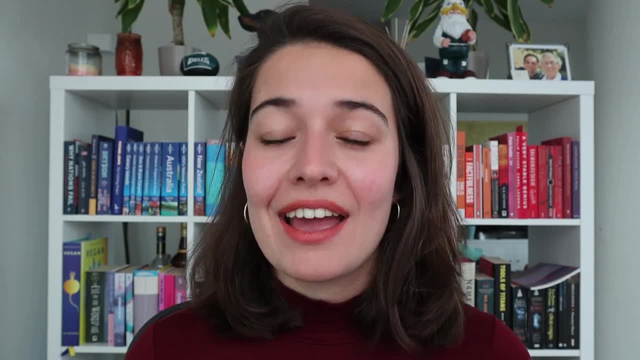 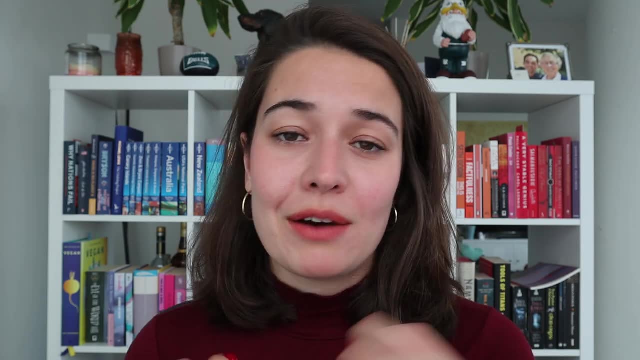 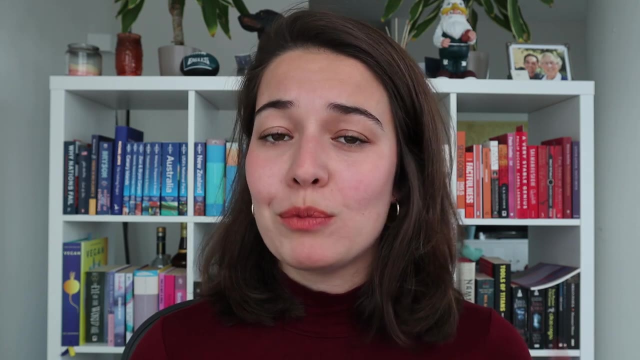 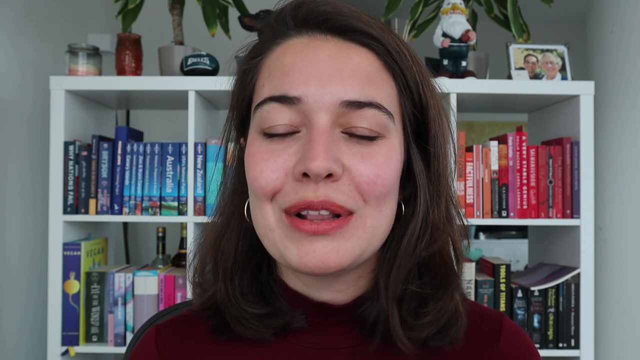 Hey, welcome back. Now it's time to look into data cleaning. I hope you're excited to fix all the problems that we discovered with the data in the previous video of data exploration. If you haven't watched that one, I would highly suggest you go watch that one. I'll leave the link somewhere here. And if you're excited about learning more from me, if you're excited about getting more training from me on data science, also go check out my course Hands on Data Science. Again, I will leave the link in the description so that you can go and learn more about it. But for now, let's get started. 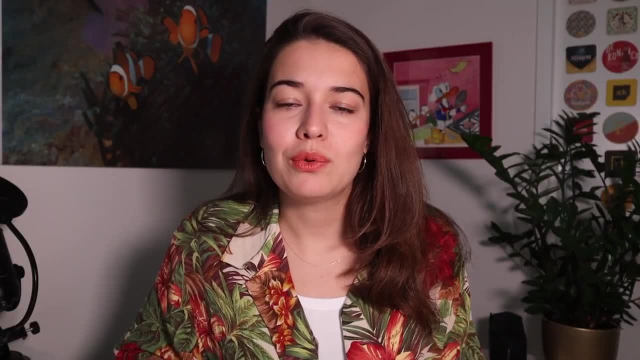 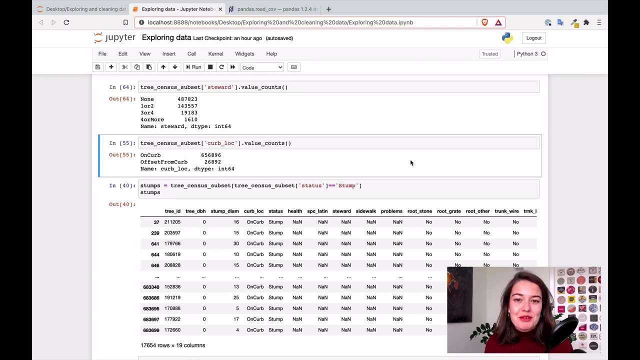 Exploring the data is actually the real deal, And I hope I gave you a good impression of how much it normally takes, because you really need to start from scratch, especially when you're working with a new data set that you've never seen before. You need to take some time to make sure that you are considering a lot of different options. You need to make sure that you're looking into what each thing is and to make sure that you're considering a lot of different options. 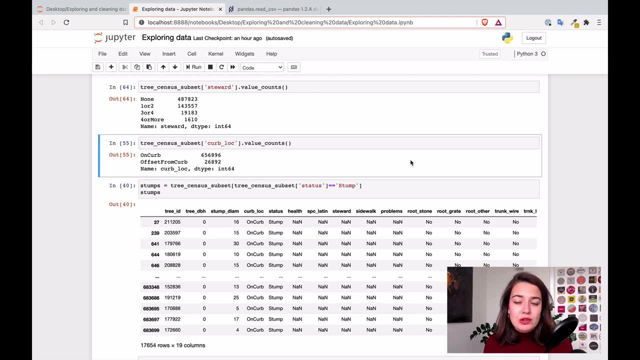 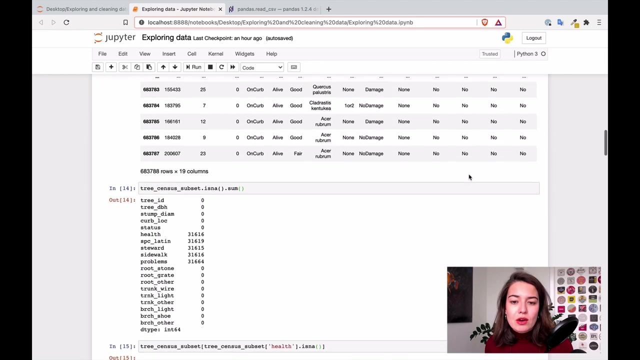 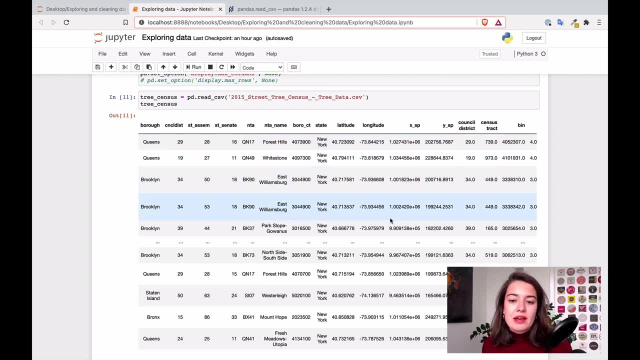 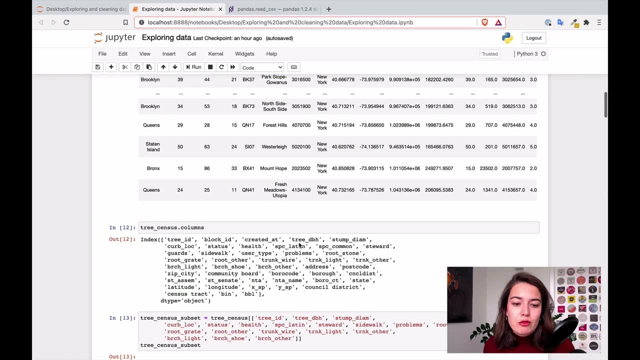 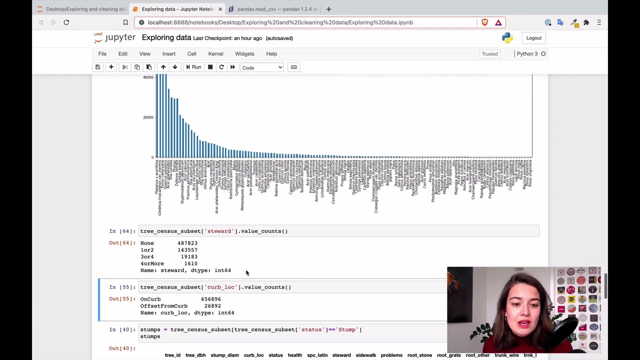 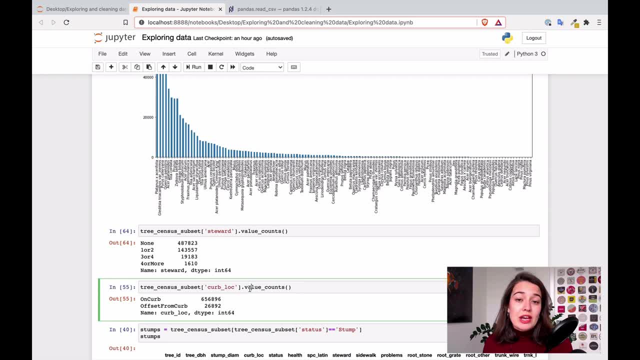 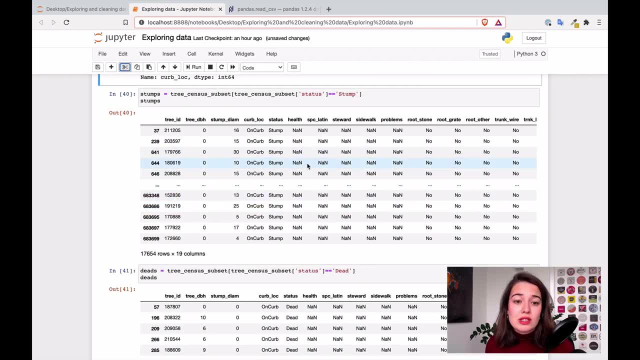 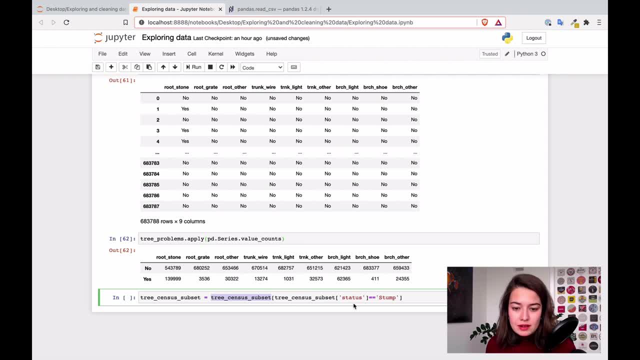 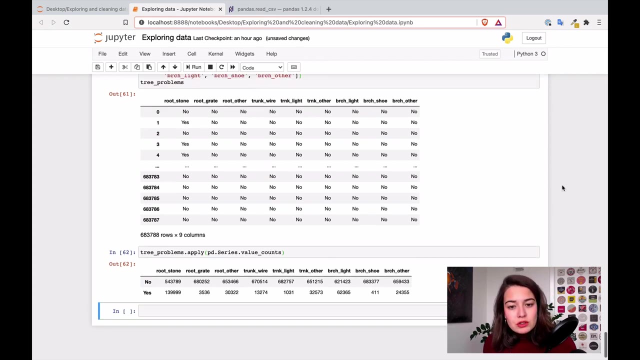 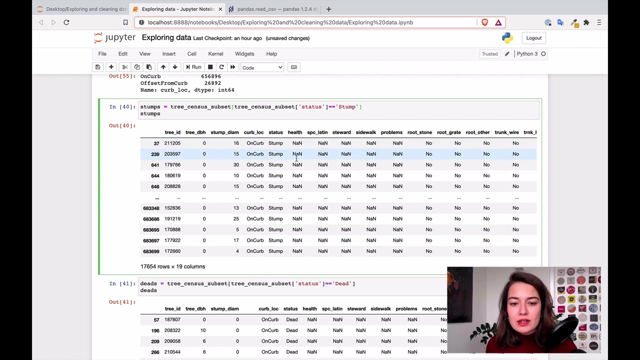 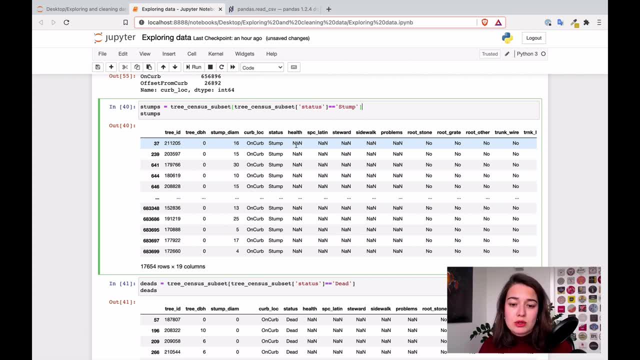 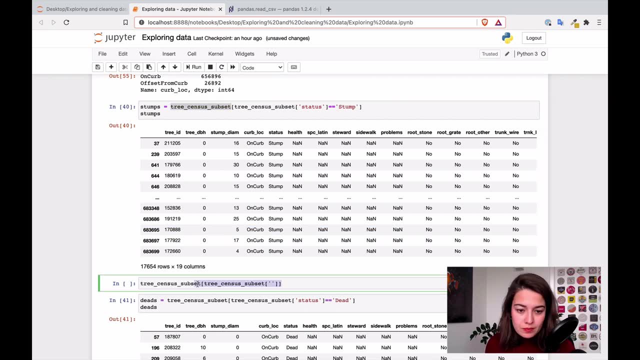 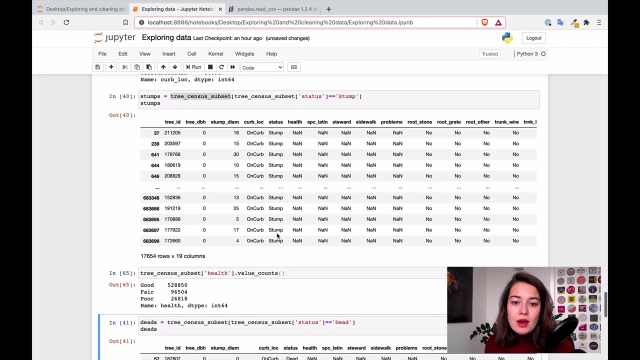 not applicable because you know they're stumps or dead, so health does not really apply to them. so if we look into it now, so basically the options for the health column is either good, fair or poor, right, but that does not apply to a stump because it's just like kind of a cut to the base of the tree. so what i'm going? 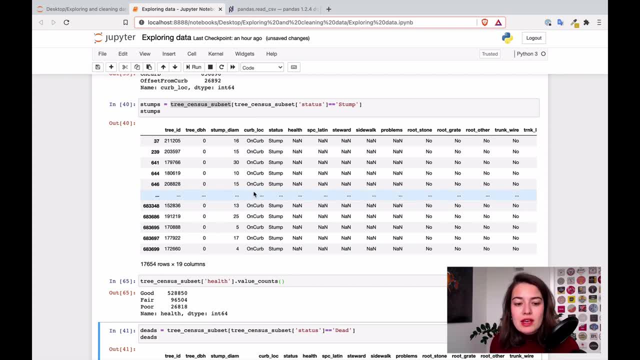 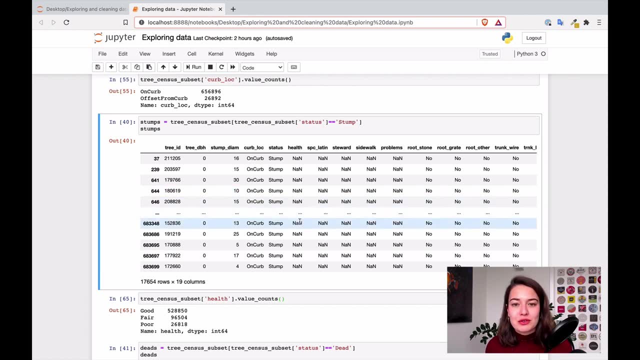 to do is add a new value here and i'm going to say it is not applicable. and what comes to my rescue, of course, to do this action is my trustable filna function, so let's do this here. uh, i mostly want to work with the tree census subset, uh, data set, so maybe let's even go all the way down. 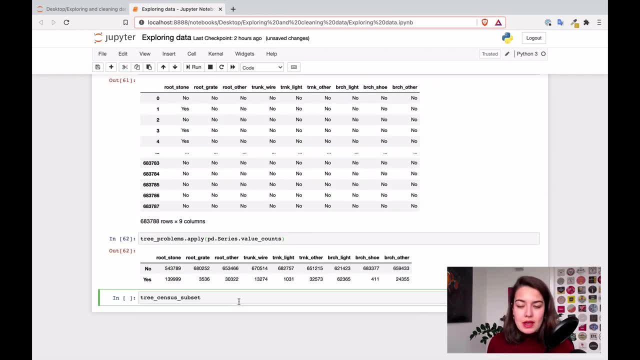 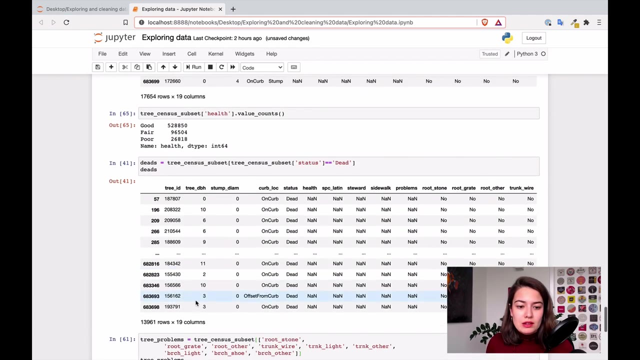 so we can work with that here. so, uh, we have the things that are stumps, we have the things that are dead trees, right, I can just say: fill now with something here, right, but as you might remember, the sum of this number and this number, so basically all the the 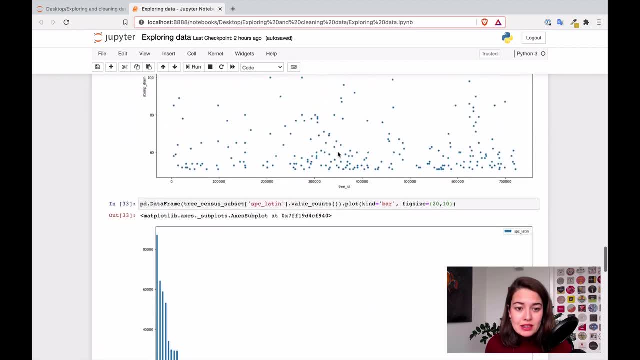 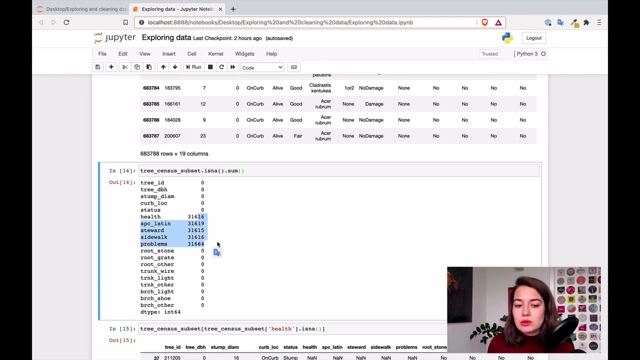 number of trees are either stumps or dead. it does not equal to the number of non-missing values that we have. there are like one or two missing ones. so there could be like, if I remember correctly, I think the the total number of that was 31,615 or something like that. 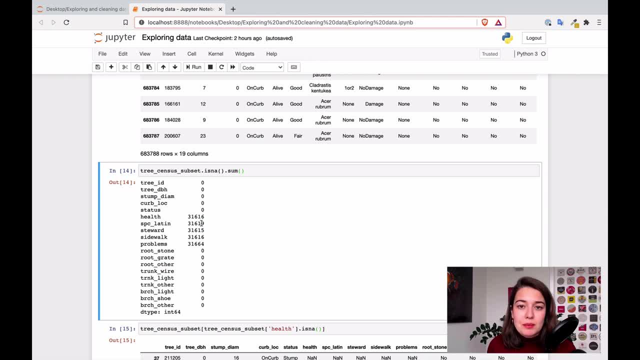 so if I fill all the non-values, I will be filling some non-values that are not either stumps or dead trees. so there could be some other non-values that I'm not covering yet. so that's why I want to be really precise and only fill in the non-values where a tree. 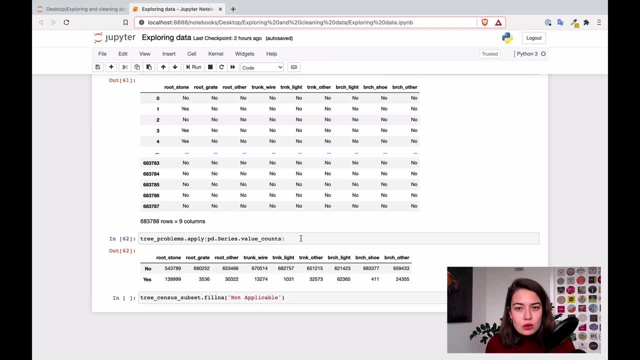 is missing. so that's why I want to be really precise and only fill in the non-values where a tree is missing, either dead or a stump, and then I want to go and see, kind of like going back to the exploration, seeing what other non-values are there are. so what I'm going to do for that is basically. 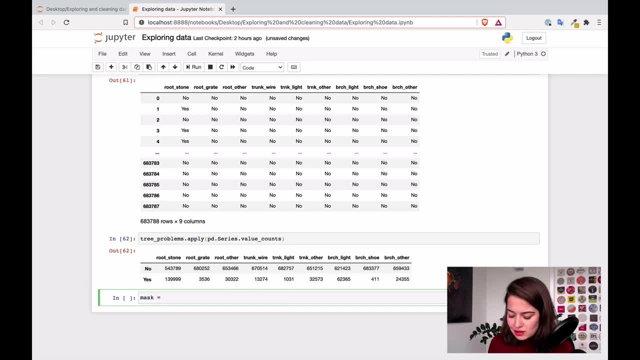 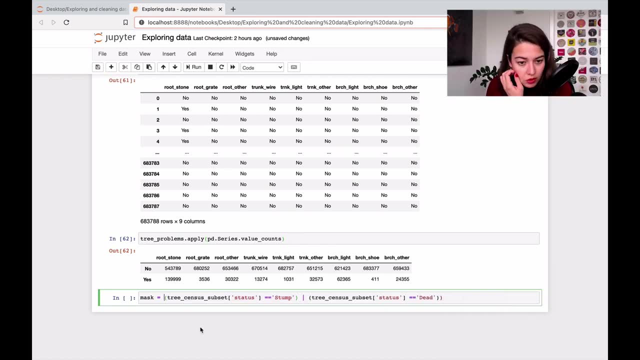 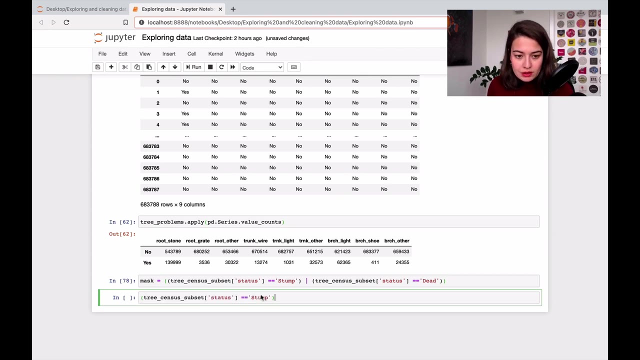 create a mask, and you'll understand what this is in a second. so basically, this mask is, you'll see how I'm using it here. I'm going to say again this, nope, not this. the data set give me all the locations, so this is like a specific way of choosing the a certain cell, basically by using the mask, I'm. 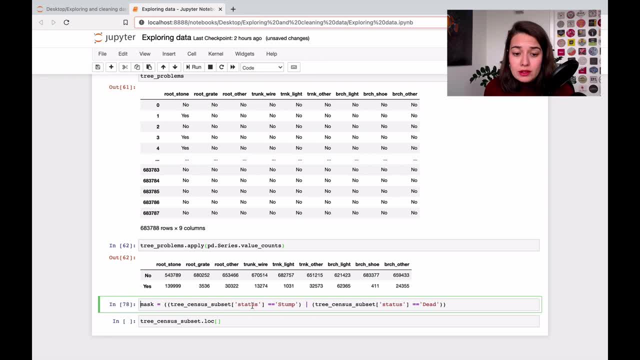 choosing certain rows. I'm saying: give me the rows where the status is equal. status is equal to stump or dead. and I will also be using the mask and I'm going to say: give me the rows where the status is equal. status is equal to stump or dead. and I will also be specifying the column that I want to update. so that's. 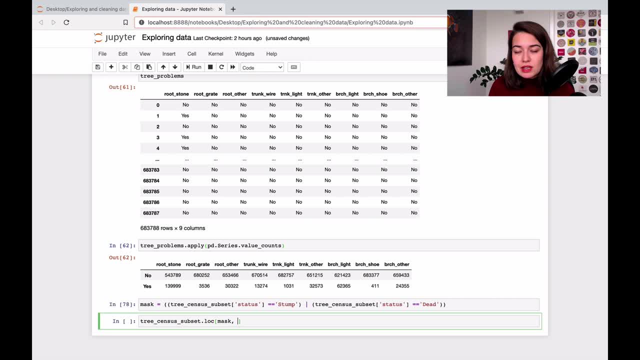 why I'm going to put mask here. so the first one specifies the road and the second one specifies the column and the column. I want health and I want to change these ones. what the same ones, but filled with, not applicable, and, as a result, I want to. 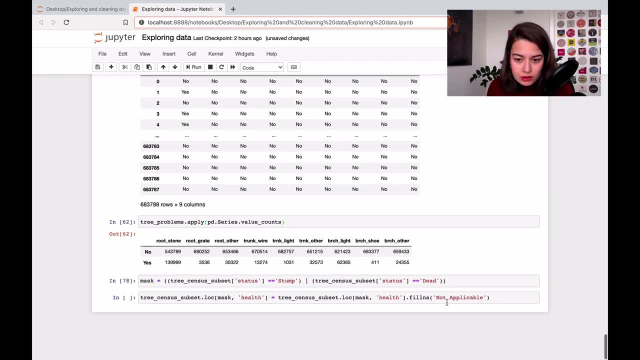 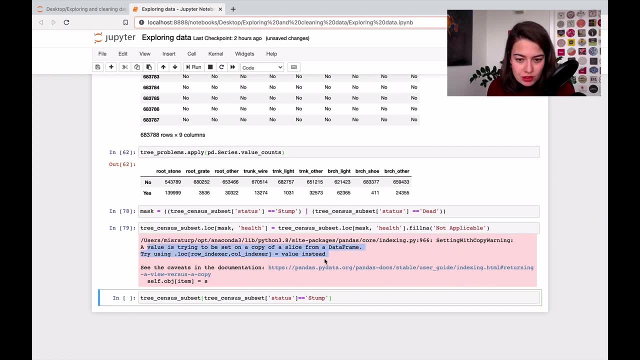 to see this one again to see if it worked or not. so, okay, it gives me a little warning here that what I'm using is not perfect, but I feel like I'm using the exact same thing, so I don't really understand these warnings. but this happened once in a while. just make sure that you're not using something. 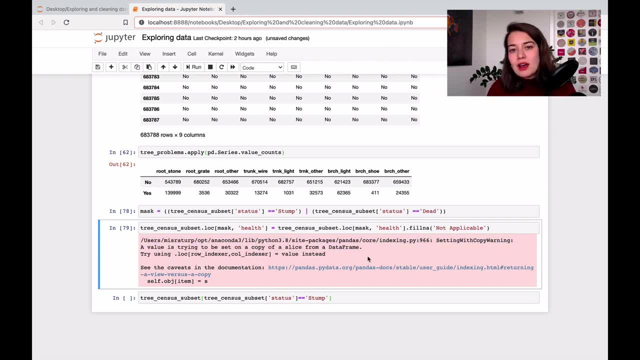 that's about to be deprecated, because then if you use it in a couple of weeks your code might not work anymore and most of the time they will give you a option of like what you should use instead. but here it says: try using dot lock, row indexer and column indexer best. 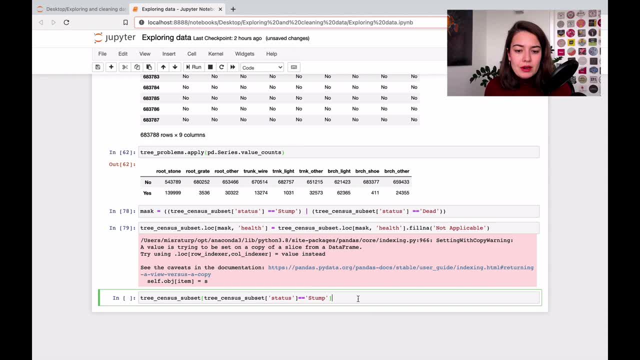 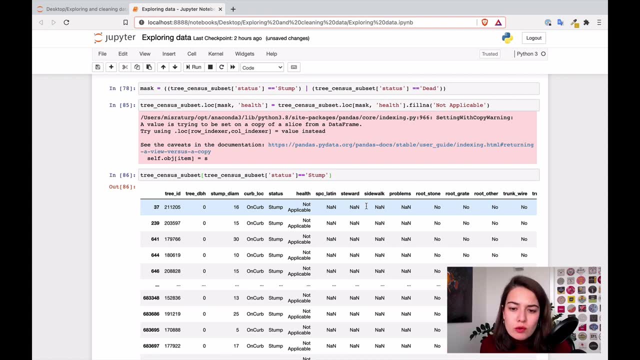 exactly what I'm using, so I don't really understand why there's a problem. but anyways, let's see, it looks like it worked. but now actually, you know, instead of going one by one here, I feel like maybe if I don't specify the column, it might still work. so let me try this. yay, it worked. okay, so now I filled. so. 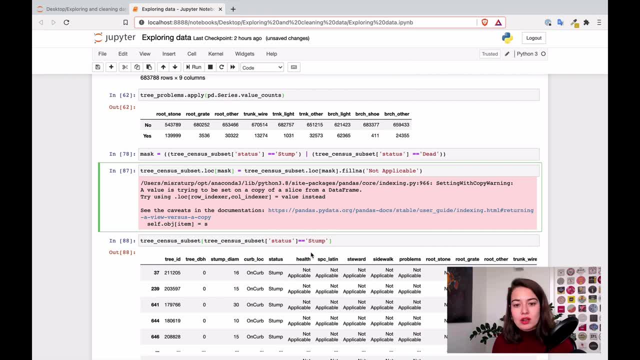 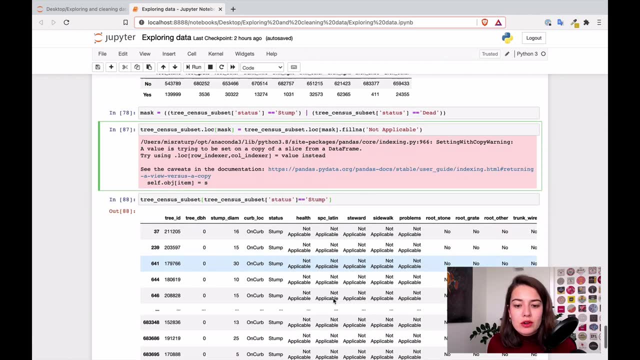 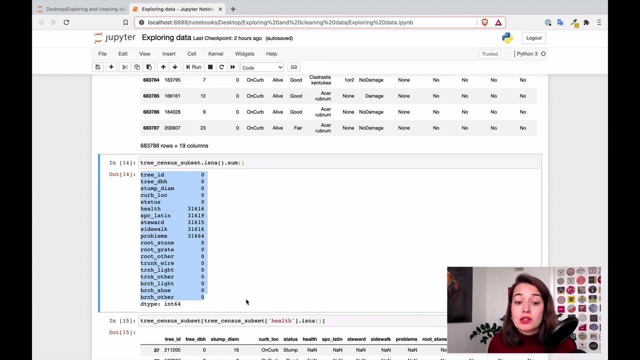 basically, I didn't specify a column and then it looked at all the columns and since I know these are the only columns where there are none values- because I've done is not that some before, as in likes this one- let me show you- yeah, I said, show me- all the counts of missing values on all the columns, and it showed me that. 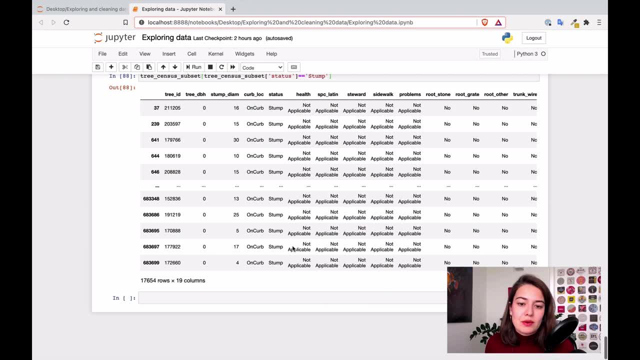 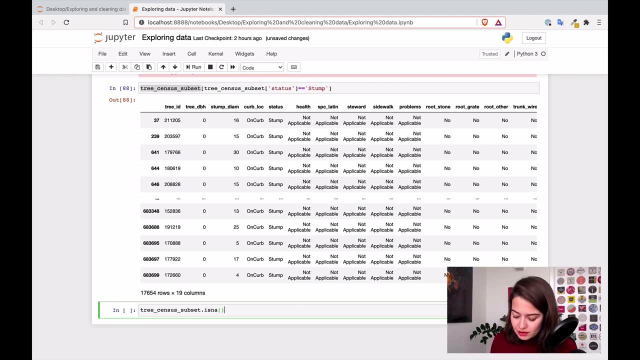 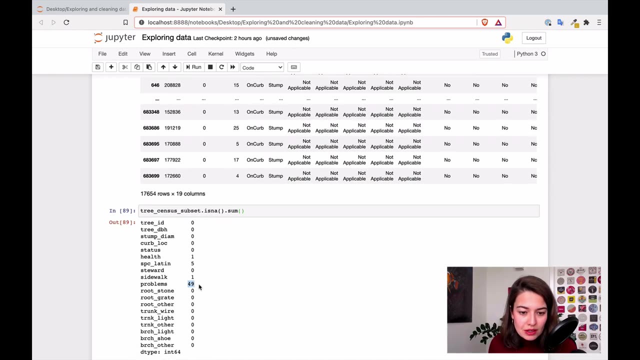 these are the only ones, so these are the only ones it could have affected anyway. so this is good to know. I still want to see if there are any other missing values, though, now that we fixed this interesting. yes, so there are 49 missing values still here, one here, five here and. 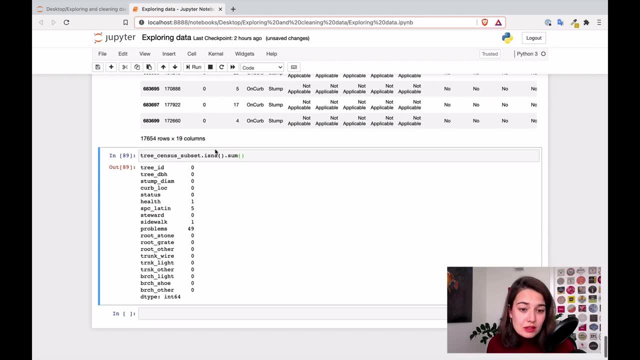 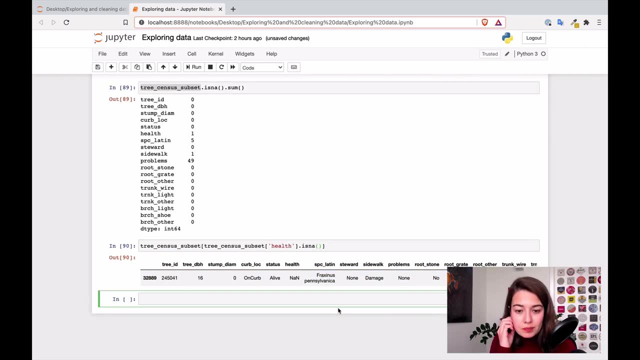 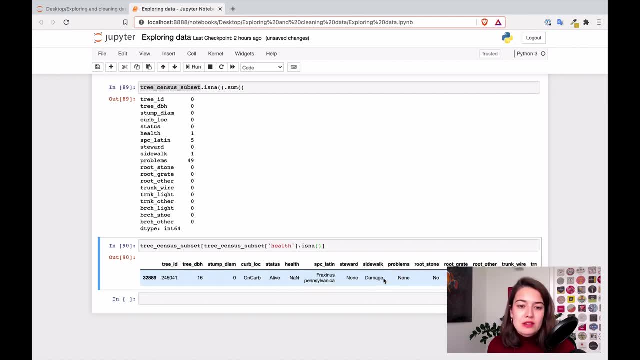 hard to know what to do with this. I think, since it's just like one value, I think it's not unreasonable to remove it, because then you'll also be removing the steward. interesting it's: a steward is not missing, but there is actually a missing value here. so let me look at the steward values. 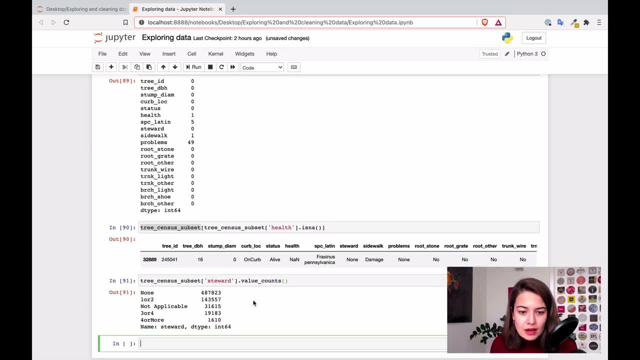 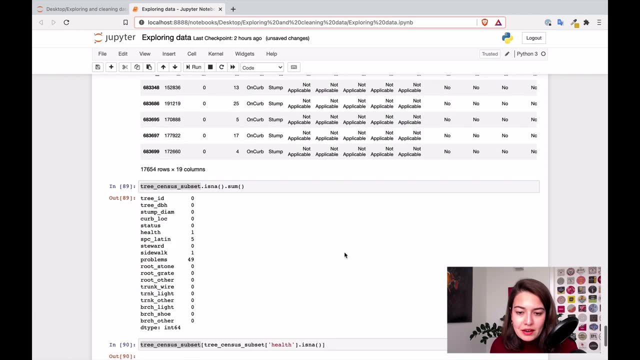 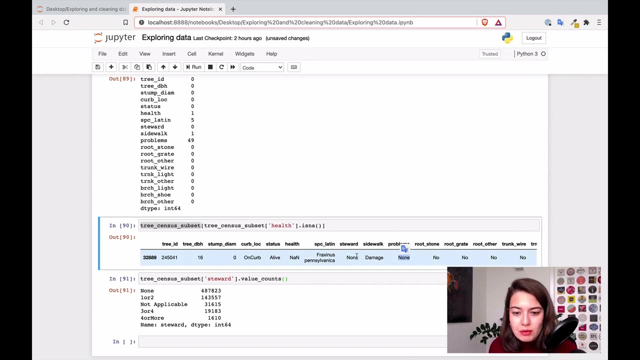 yes, none, I guess. okay, in this case, I think none here. it's not like the NAND that we've seen before, like not a number. I think none here means yeah, it just does not exist there, there are no problems and yeah, problems, or there is no steward, so okay, that that's not the none that we're looking. 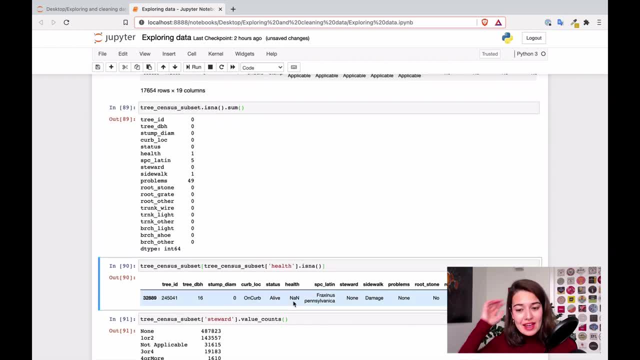 for it's not the missing value. health is NAND, though, so it's really hard to decide then. on that case, I would probably just remove this one, so let's look at the sidewalk one. I mean probably the sidewalk one. I mean probably the sidewalk one, I mean probably the. 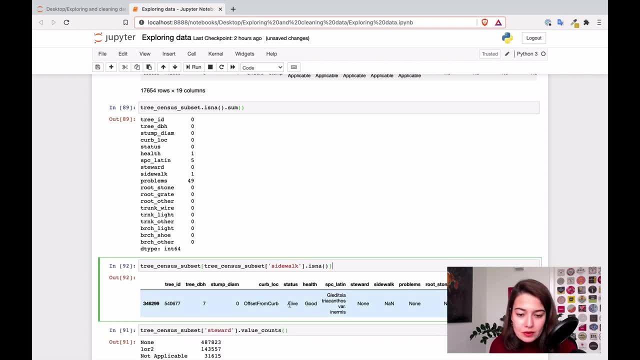 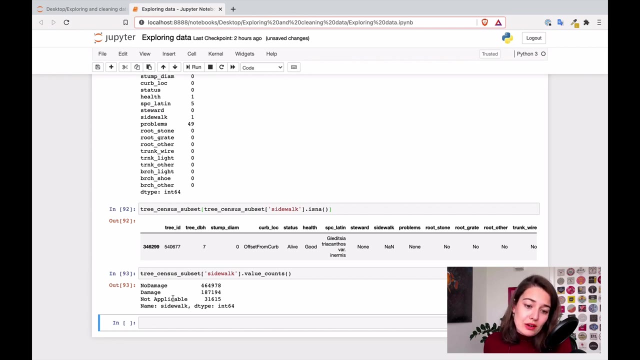 same. to be honest, alive, health, good sidewalk, NAND and values for sidewalk is no damage, damaged not applicable. what created not applicable. so I would probably actually, since these are just like one values and they cannot affect the outcome too much and we might want to keep the other values, like you know, I might want to delegate that into other values and they can't stay they were not Ganon values since the � november sprinta knife from this is cocoa and they cannot affect the outcome too much and we might want to keep the other values like you know I might want to do that and then I else above. it has four vertex. does that say they are non non deals in the presentation. but why would that essentially be an additional value area first, or it's a non non for Shelley. so I would Python go ahead and I'll look at the original solution. so I 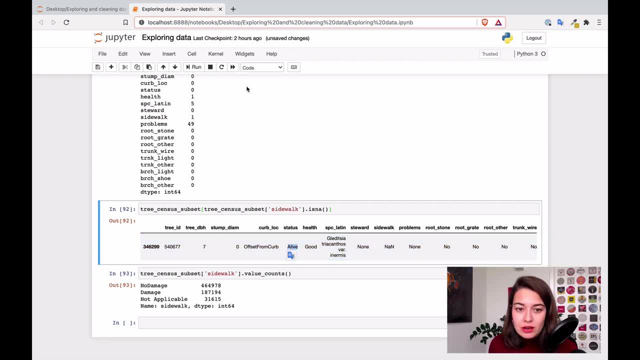 to know the actual count of how many alive trees there are. i actually i changed my mind about the previous missing value too. i would just fill it with whatever is um the most common value here, and i think no damage is the most common value. so instead of 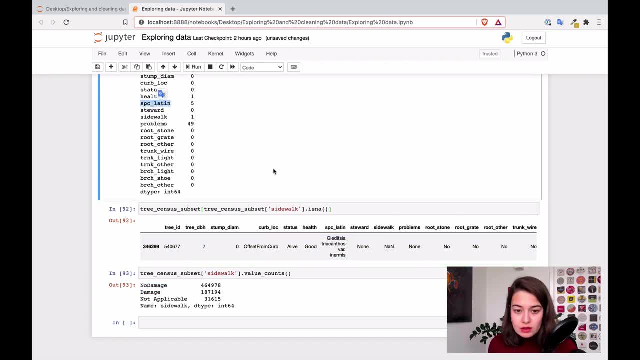 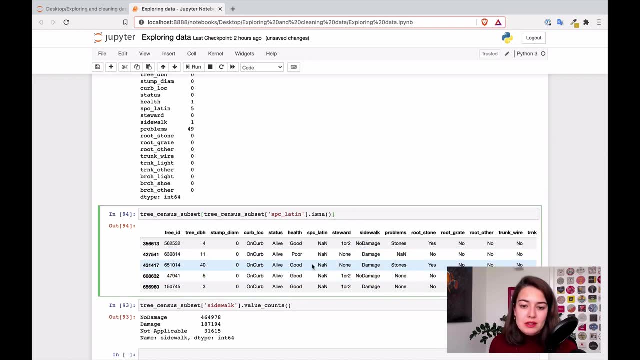 none here, i'll just have that one. so let's also look at this one. this is a little bit trickier um, because there are five of them and also this is like. it's not like if the tree is healthy, if there are problems with it or not. this is like the type of tree. so 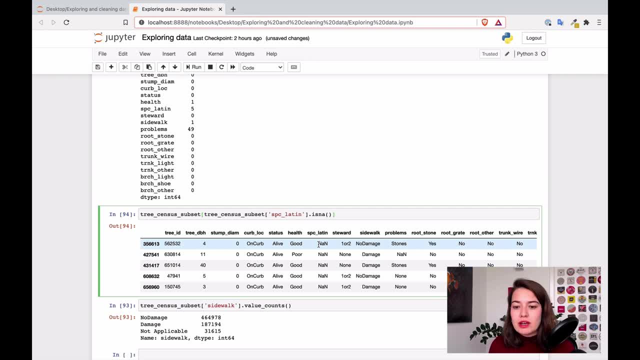 instead of the type of tree here, i think i might put like, uh, i'll just say like couldn't observe, or something like that, and i'll fill it with like couldn't observe, um, we'll look at those ones, and then let's see problems. um, um. 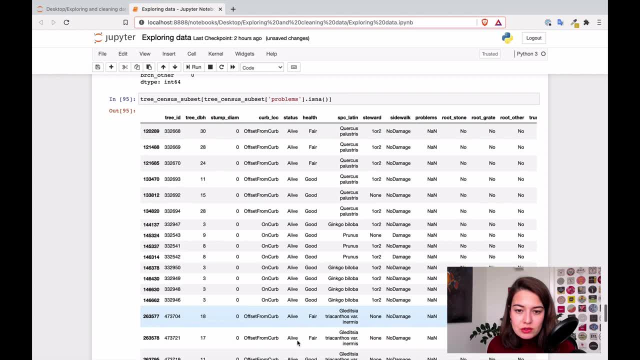 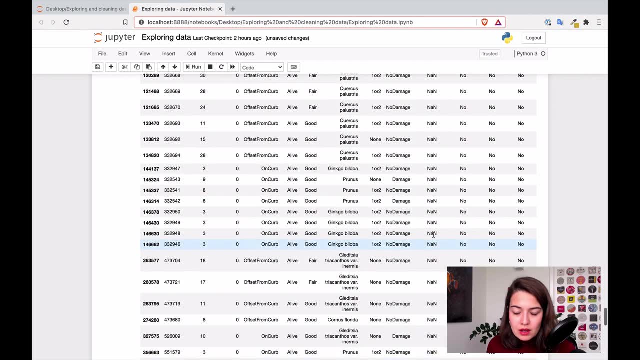 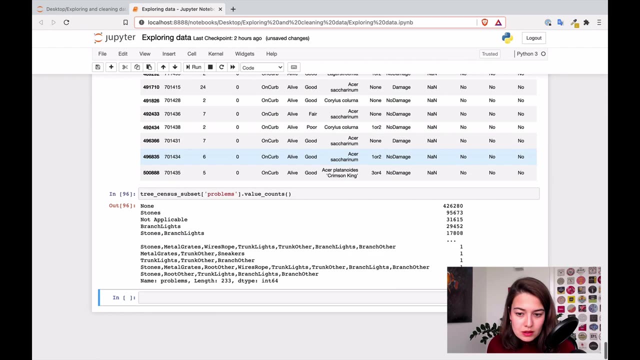 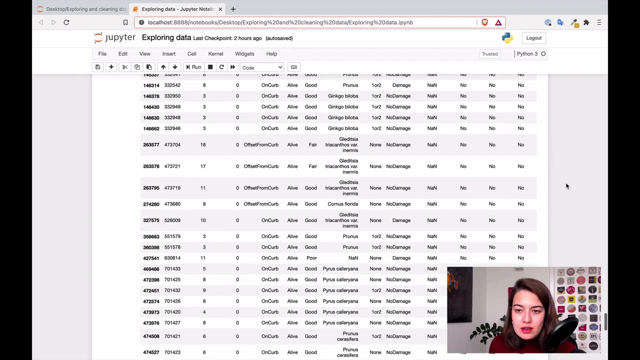 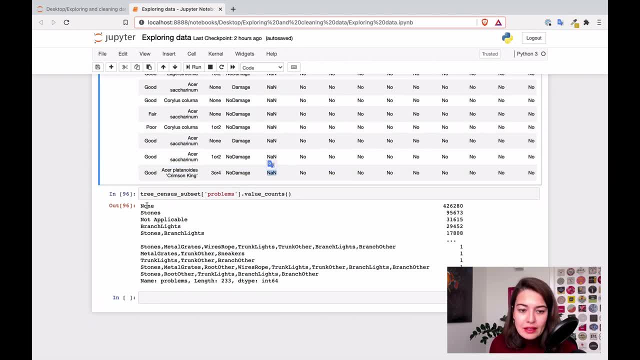 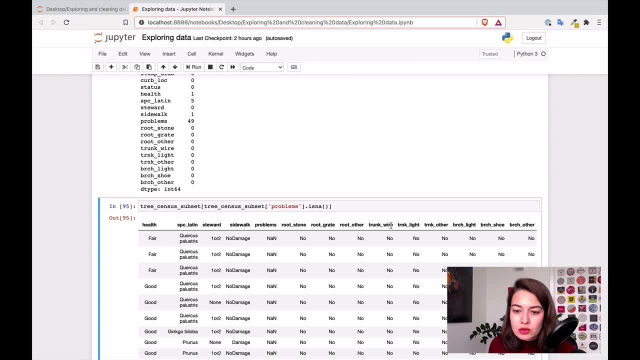 none this way, so i'm going to fill in the problems with none this way, so i'm going to fill in the one. so, instead of like, not a number, i think we can fill it with just none, because, you know, these are the problems that there would be with, like, the root or the trunk or the branch, and these are all nose. 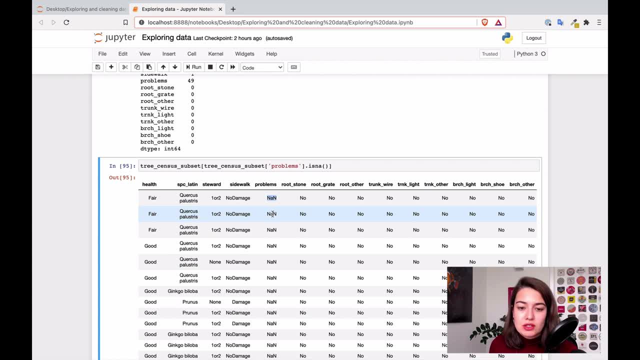 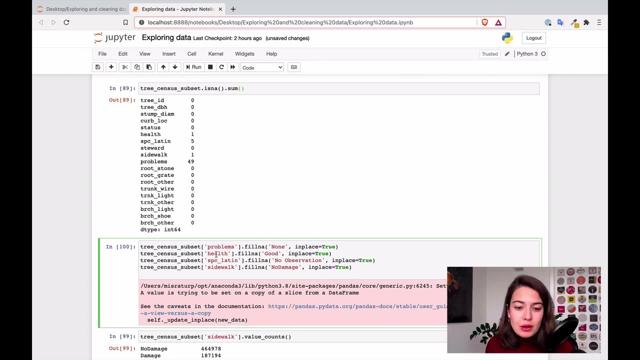 so i think it's fair to fill these with uh, just none, uh. so let me do all of these things and i'll meet you back here in a couple of seconds. all right? i quickly checked what the most common values are for problems, i'm sorry, not problems. 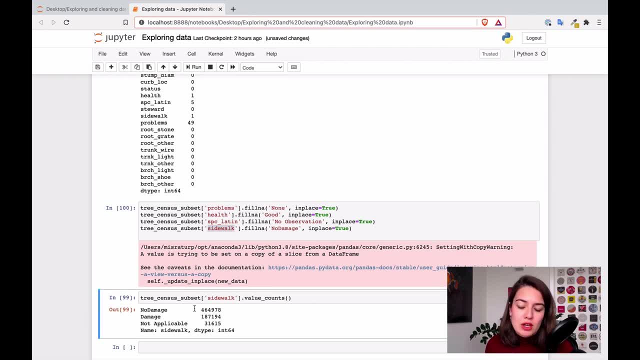 health and sidewalk. just using the value counts and looks like the most common value is for sidewalk- no damage. so that's what i assigned to the missing value. uh, for health, the most common value was good but, as i said, these are not going to be like valid data points, but it's like one data point. 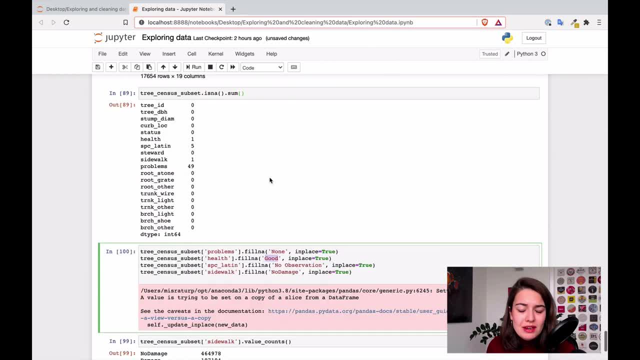 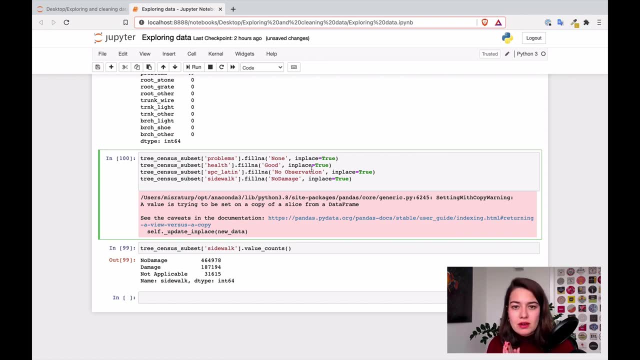 out of like what was that? like 60 000 or something like that. so i think it's uh, yeah, it just makes sense uh to just like just to keep the other values uh in our data set. i think it's worth it. we're kind of like lying a little bit like a white lie that will help people. 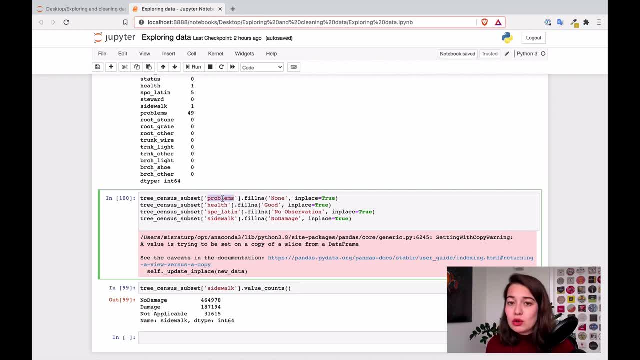 um, problems, as we observed, it looks like there were no problems, so we can easily put none. i think that is accurate and for the latin, i'm just creating a new value instead of the name of the tree. i'm just going to say no observation, you know, it's just, or something similar. so if i try to see, 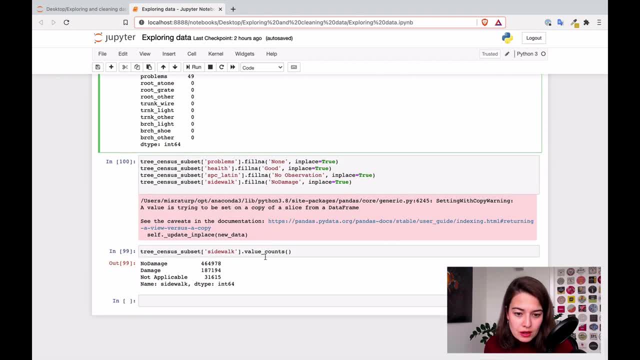 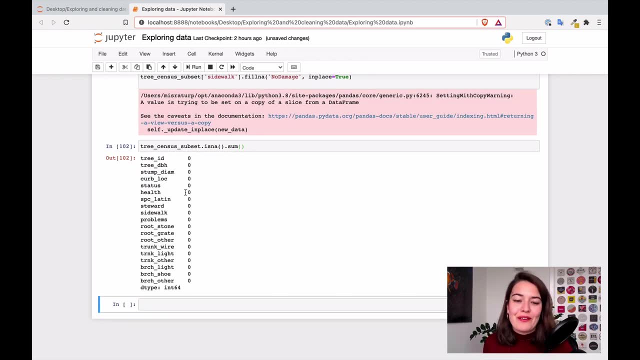 how many missing values there are. again, just keep the kind of thing running here. let me put it here: no more missing values. so you. that's great. finally, we cleaned our data, uh- from the missing values, and there is one last thing that we need to do, and that is to deal with the outliers that we figured out before while we were. 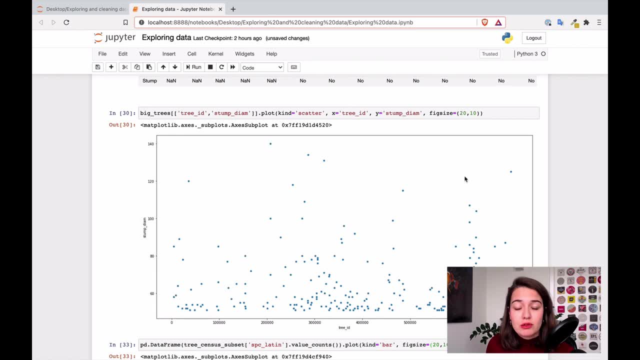 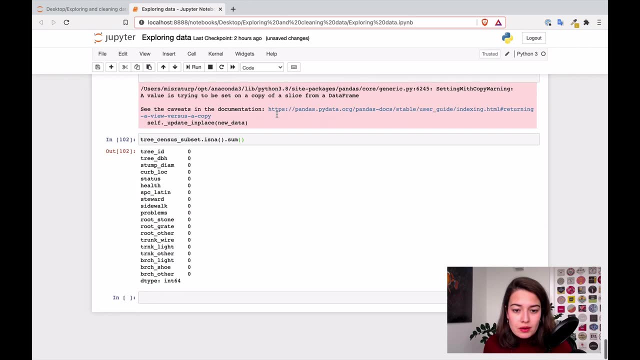 exploring the data, and those are the ones that we saw from the diameter, um. so yeah, let's, let's, let's look at those. we already said these are the big trees. i think i'm also going to include the other uh values, like so: either the stump diameter is higher than 50. we said 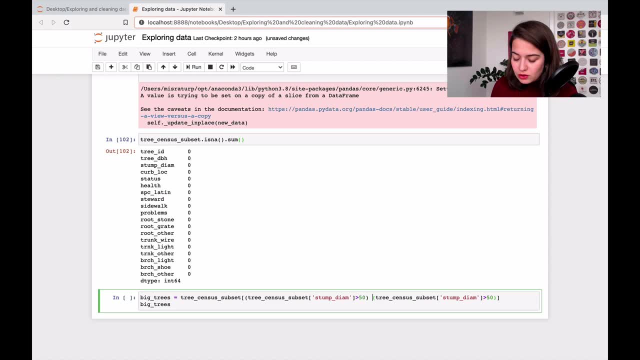 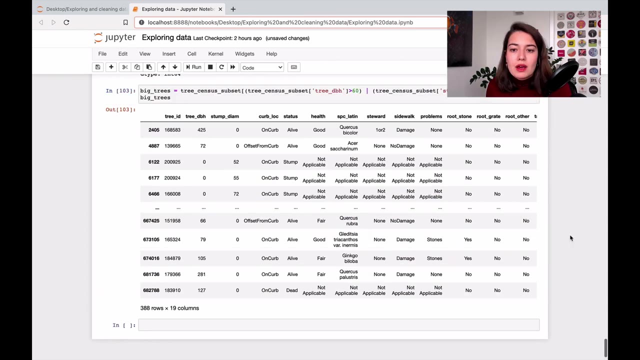 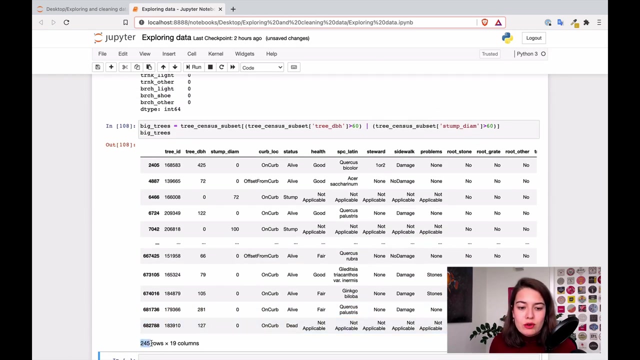 or um. the tree diameter is bigger than 60, was it? i'll just go check it again, but i think it was something like this, right, um? so yeah, let's keep both on 60.. so this is, uh, the tree. so now we only have 245 out of. 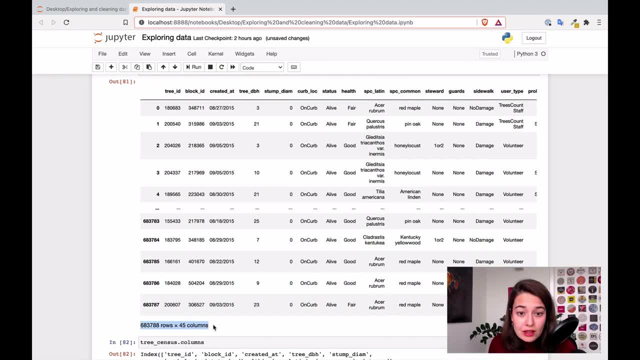 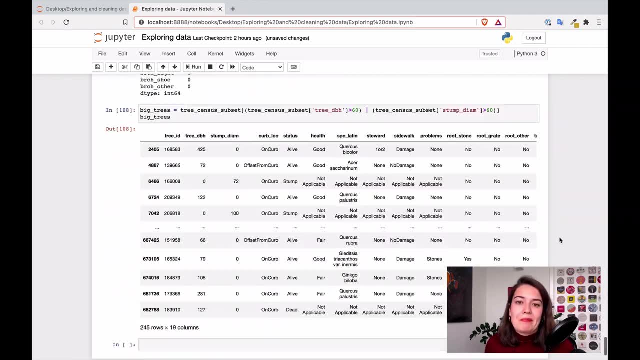 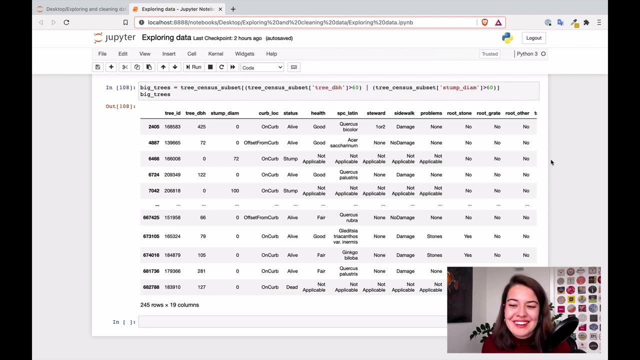 a total of, by the way, as you can see here, you can see that we have a total of the number of rows and columns 683 000, nearly 684 000, so not a lot of outliers. one thing you can do is just to say you know what, i'm not interested in these, and just like cut them out. that's totally. 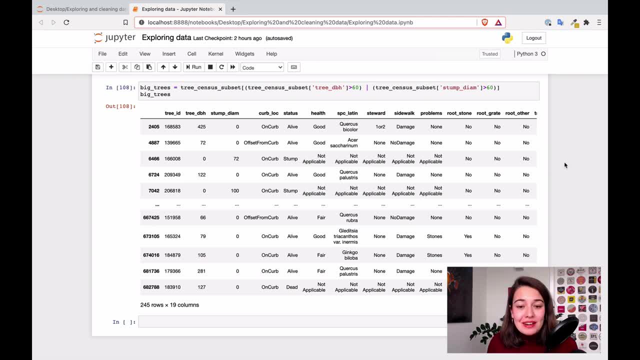 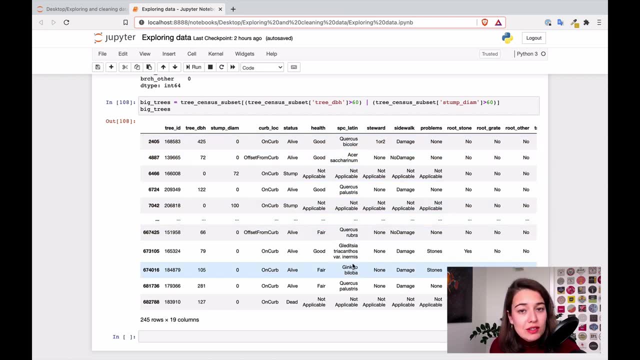 acceptable way of doing it, uh, but another way that we can do this, which i think could be like an interesting exercise, is to see what type of trees these are and either get the average value value, uh, from this of diameter for these tree types from the original data set, or, like the 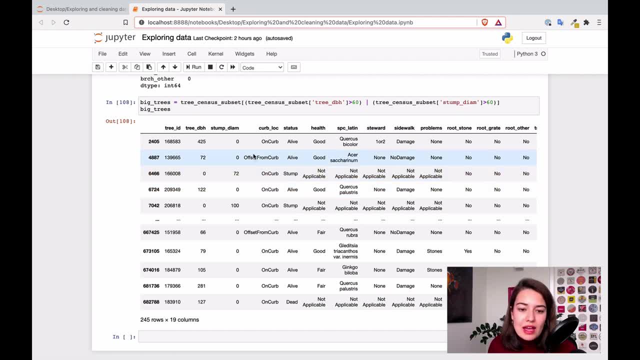 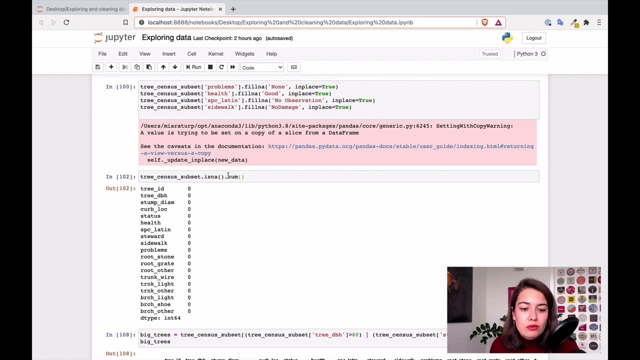 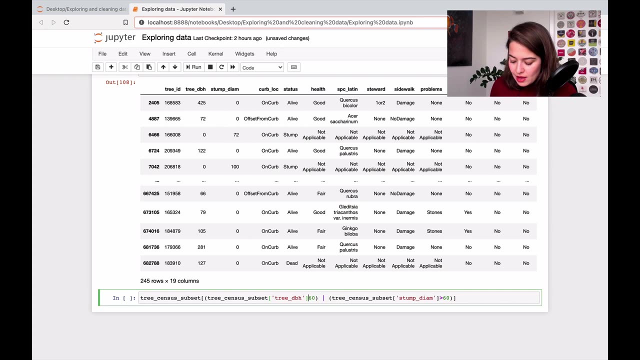 maximum value maybe, and change the diameter here with that. so that's one thing we can do for that. what i want to do is actually first remove those trees from the original data set that that are a little bit too big, too big. so i'm going to say trees need to be either equal to the tree diameter. 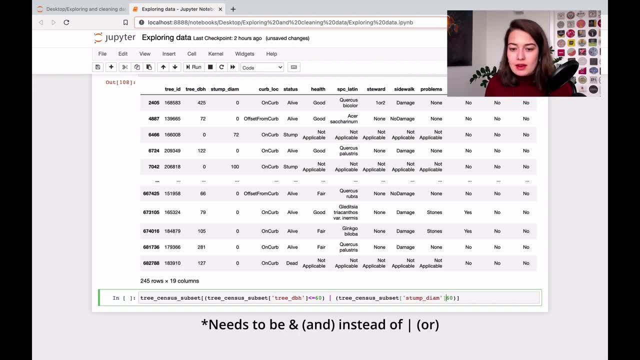 needs to be equal to or less than 60. so i'm going to say trees need to be equal to or less than 60. and again here, also, the stump diameter needs to be equal to or less than 60. and i am filtering the original data set. so the reason that i'm doing this is because if i want to calculate, 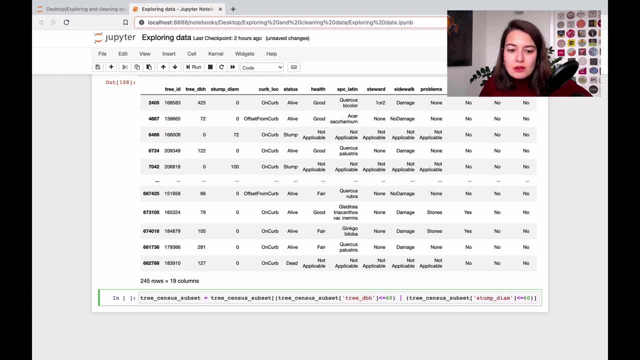 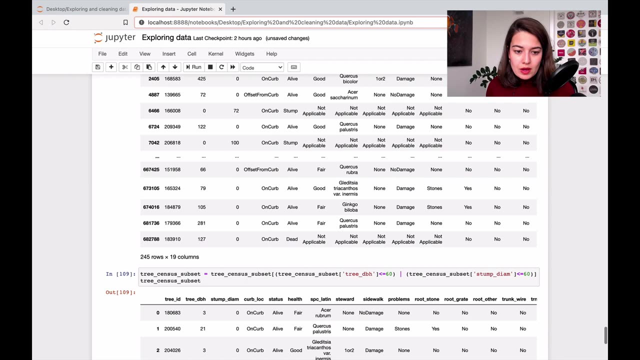 the mean centimeter for the trees and the mean diameter for the trees. i don't want to have the outlier information there too, because it's going to affect the mean that i'm calculating. um, so let's do that, okay. and i also want to have the alive and the dead trees separate, or like stump, and 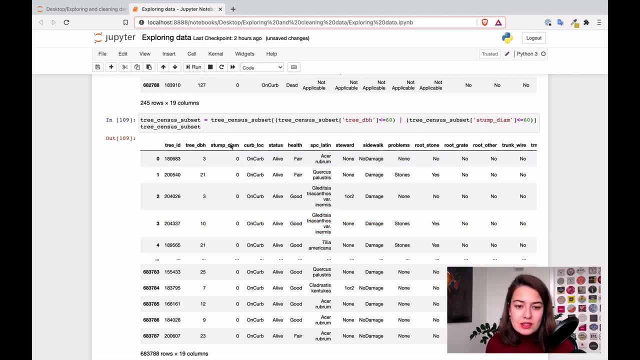 that tree separate because, uh, as you can see, if a tree is alive, then the stump diameter is zero, which is actually not the case. it's just that they just didn't calculate it because it's not a stamp, it's an actual tree. so then i want to have a separate um data set for stump and or stump or. 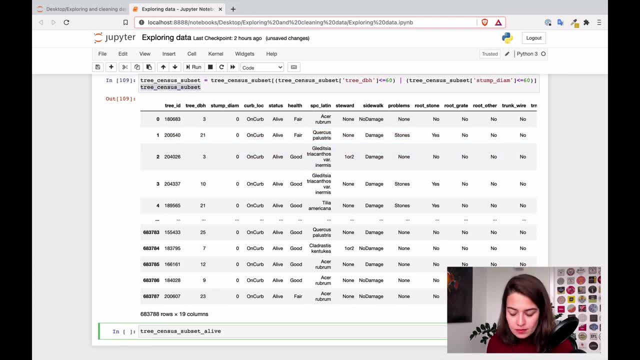 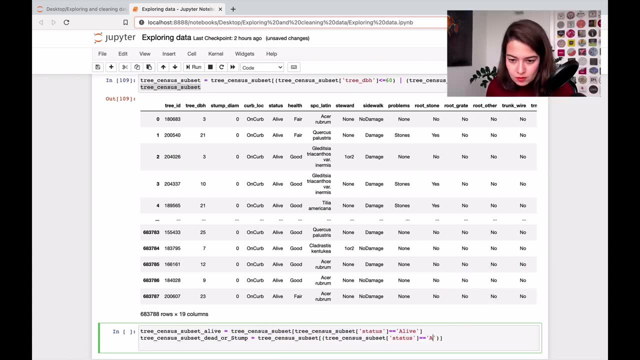 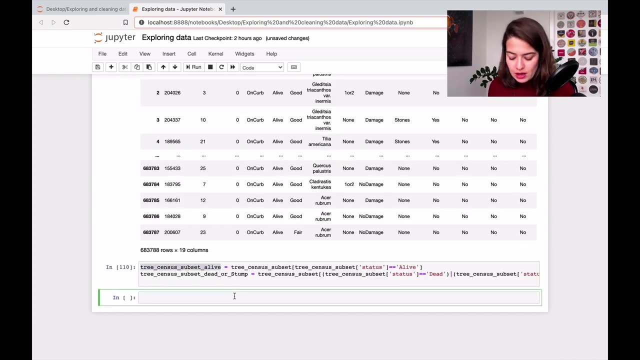 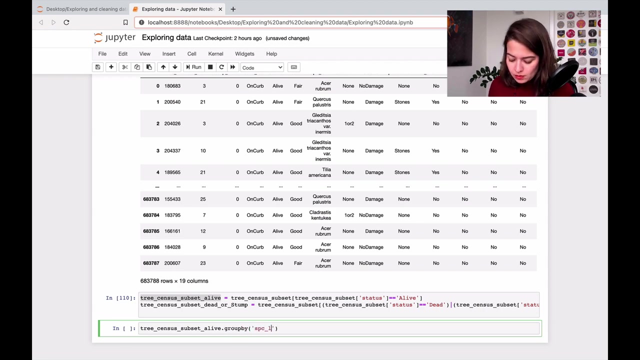 dead or alive trees. is it a tree? that is a tree. is it a typeets? are you a tree? is a typeets? asked: what is a tree? okay, now that i have those, i am going to group them by the tree type. okay, so this gives me for each. 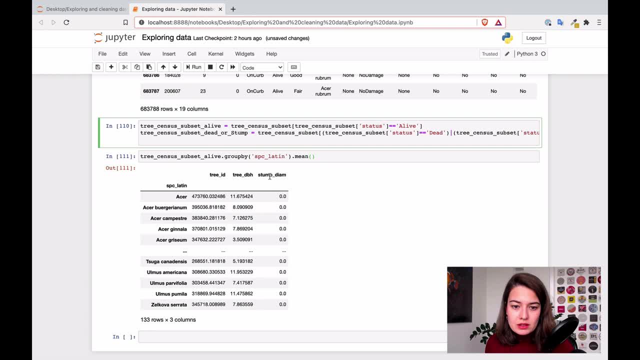 le, tree species, the stump diameter and tree well, which is 0, because this is only for the alive trees and the tree diameter. the tree idea, as I said again, I should have changed it to string all the way at the beginning. I think that would have been. 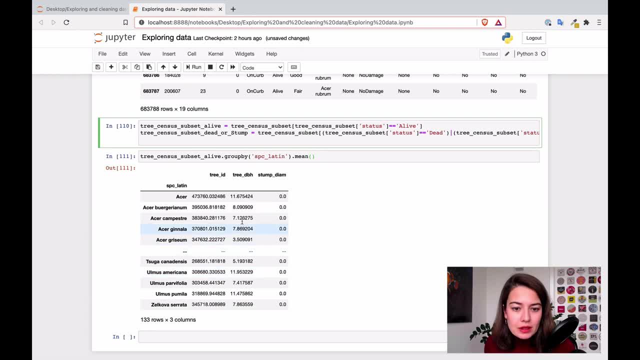 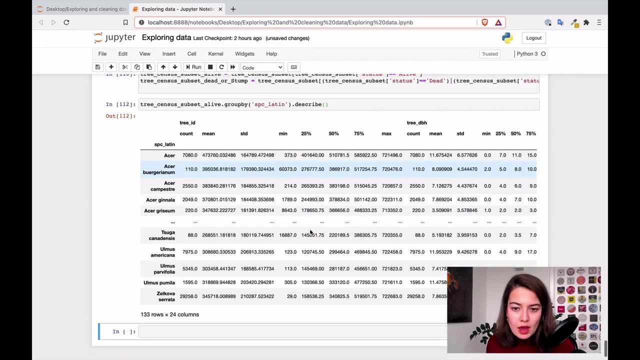 useful so it doesn't keep popping up. yeah, so these are the values, so this is just the mean one. if you want, you can also use the maximum, but or the minimum or 25th percentile value, I guess. yeah, this will also give me all the information when it comes to. 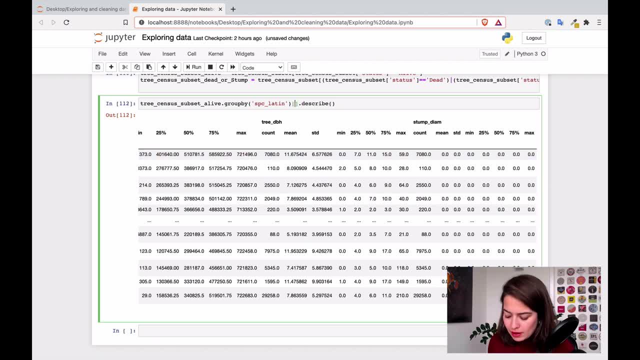 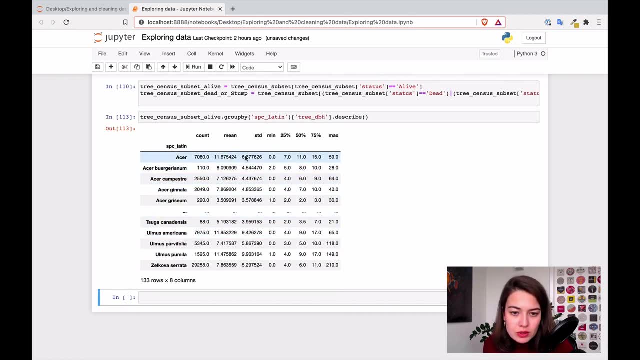 tree. maybe I can even specify what I want. okay, that's better. so for each one, the mean standard deviation, which is not very high. well, I mean, in the examples that I'm seeing, which is good, the minimum value and the maximum value. it's a bit weird that it's zero. 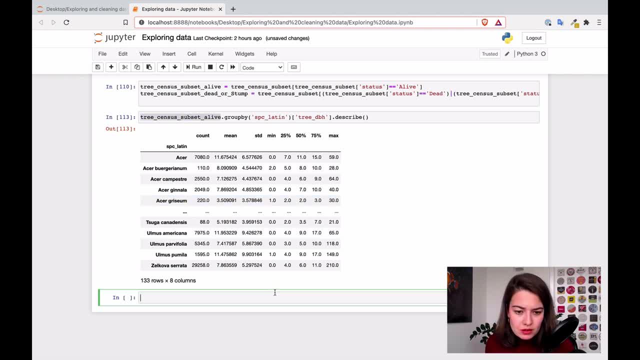 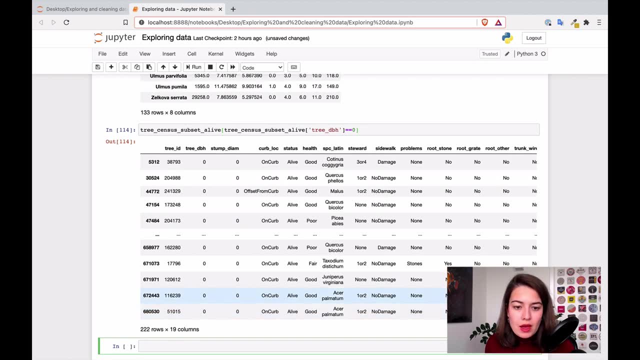 to be honest and maximum value, want to see the ones that are zero, which I feel like shouldn't be happening. hmm, okay, I feel like we're now kind of while trying to fix something that we explored before we actually found something new. that is interesting. 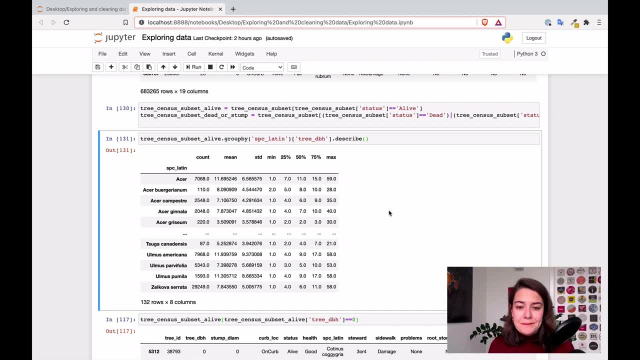 so I think at this point we have a front of us. i have two options. either i'll just go forward with only um, changing the values that look a little bit too high and the values that look extremely low, like zero, which like doesn't exist, or i can say you know what? actually? everything that is bigger than the 75th percentile. 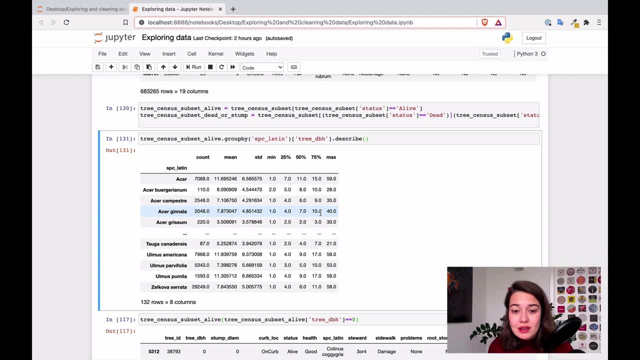 value of this tree is too big, so i want to kind of like shrink it down. so if the maximum value is 35, that's actually just probably mistaken. it should be lower and it should be nine, and everything that's lower than four is probably was probably a mistake. so i'm going to bring it to all the way. 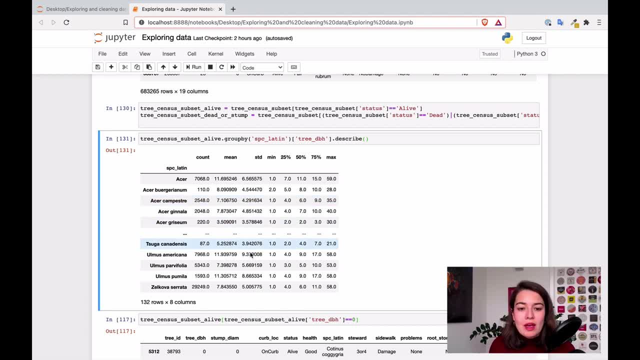 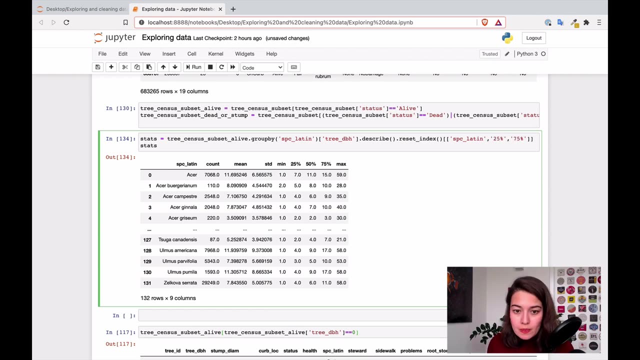 to four, so i'm going to show you the second one, just because it's a little bit more fun. um, so i will take this list as a reference, and i'm not going to do it for the dead trees, because if you remember the names of the trees, 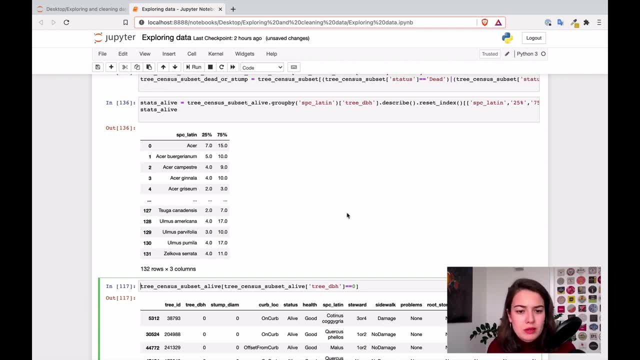 were not even written. so we we said like no, not observed, or something like that, so we don't need to do that, so just need to do this for the alive trees. so how i'm going to do that is: i'm going to actually merge. i can delete this one. i'm going to merge this new table that i created with the. 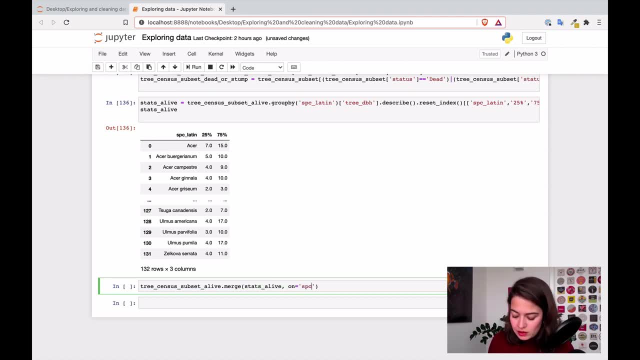 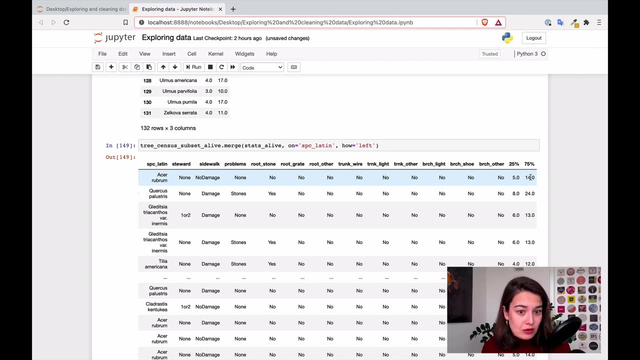 one that we already have. okay, so we have the diameter of the tree and we have the minimum and the maximum diameter of the tree, so what i'm going to do now is just is to compare it to the minimum and the maximum and if if it's lower or higher than that, i'm going to bring it to that limit. 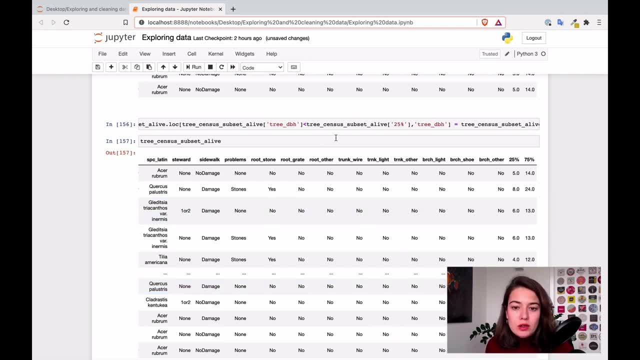 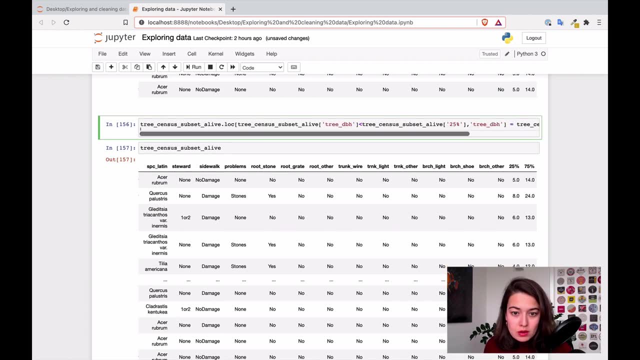 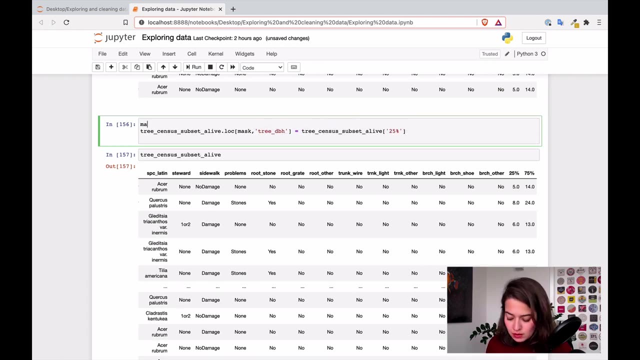 yeah, so for the lower one i've already done it, so this is kind of like we can make this a mask too. oops, you know, i'm just saying this. this is the condition, and when this condition holds true- as in the diameter is lower than the lower limit, then 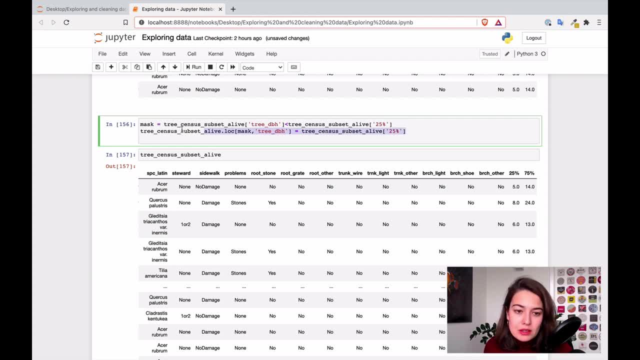 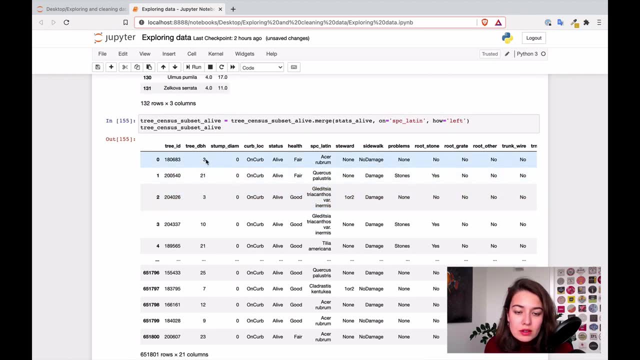 make the tree diameter equal to the lower limit, and then i'm going to bring it to the minimum limit. so i'll i'll do the same thing for the higher limit too. so you know, you can see here, the lower the tree diameter was three, but actually the lower. the lowest we decided it could be is five. 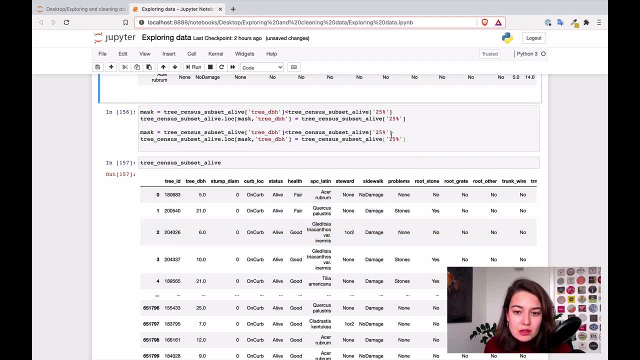 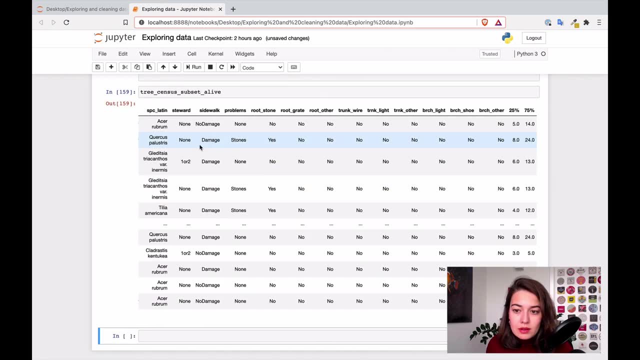 then i changed it and now this value is five. so i can do the same thing for the other one and let's see now the. was there any that was too big here? maybe this one? yeah, so i'm going to bring it to the minimum and then i'm going to bring it to the maximum. 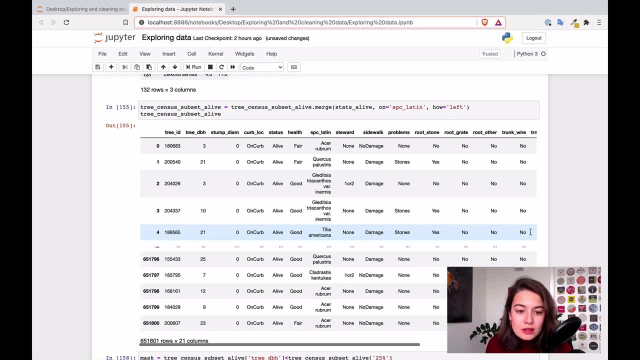 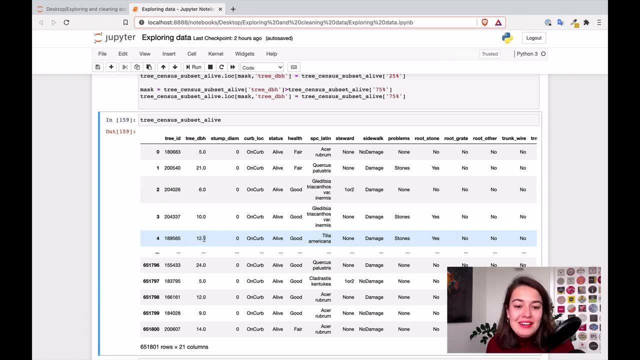 yeah, so this one was 21, but we said the highest it could be is 12.. this is the fourth row and now it's 12, so it looks like we did a good job cleaning it. uh, yeah, so i've already cleaned the alive trees. if you want, you can also clean the trees. you can say oh no, but like if, even if they're. 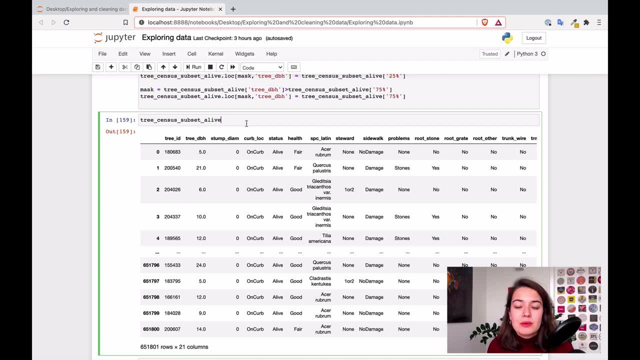 dead. they cannot be zero. you can make them higher, but the problem is we don't have the latin names, let the species names for those trees. uh, so one option could be to delete the ones, that where the values are zero for the dead ones, or, um, yeah, you can just get like an average. 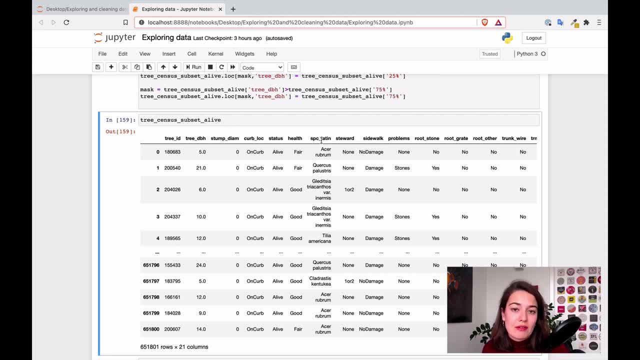 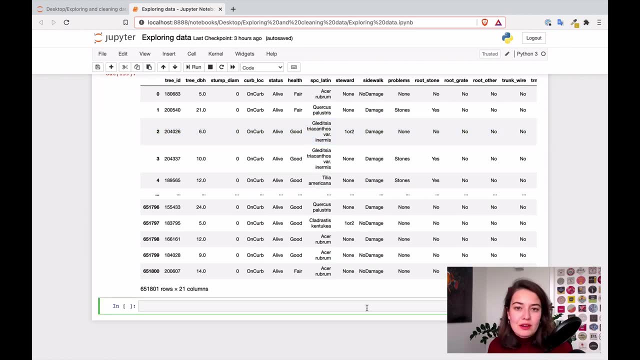 a number for the trees if you really want to keep those data values, data points and then keep them in a database. but this has been a really long-winded way of explaining how we can do data cleaning, um, but these are basically all the steps that you can do. one thing that i 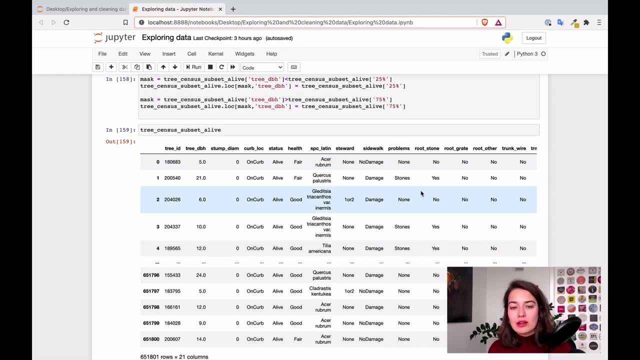 want to mention is that if you do not have a lot of problematic data points where they're like outliers and stuff, you can actually, even, like, pay special attention to it if that data point is really valuable to you. let's say, we only had one outlier, like you know everyone, everything was more or less on the same level, and then you had one that. 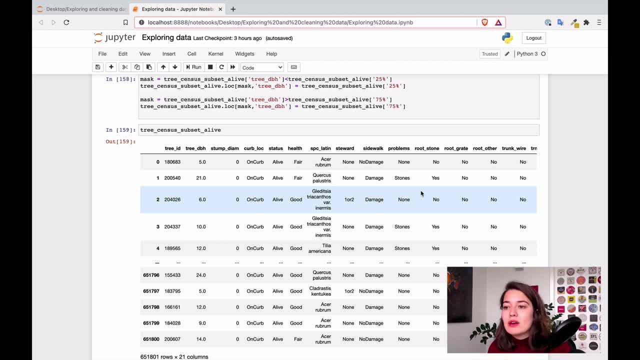 was like 500 inches, then you can look into it, maybe. okay, then you can think, normally this trees diameter is between, let's say, 25 and 55, so maybe this person was trying to type in 50 and then they accidentally put 50, 500 and then change to 50. so 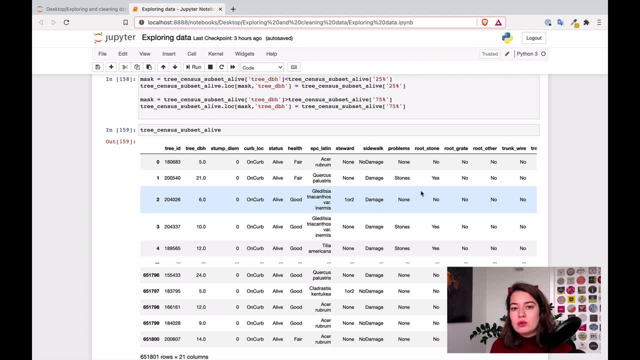 if they don't have a lot of problematic data points, they can actually keep them in a database. data points are very important to you and you um want to fix. if there are not a lot of problematic data points- let's say they're like three or five or something like that- then you can pay special. 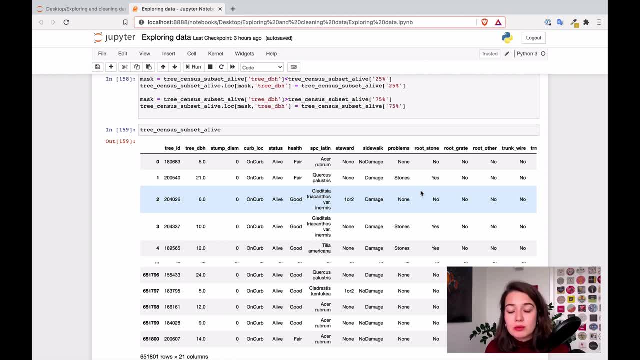 attention to them and then go one by one and find the most reasonable solution. but when you have hundreds of them, like we did here- and we generally have a lot of data points- they're not necessarily extremely important to us. i think that the best way is to automate them, so i hope this was helpful. 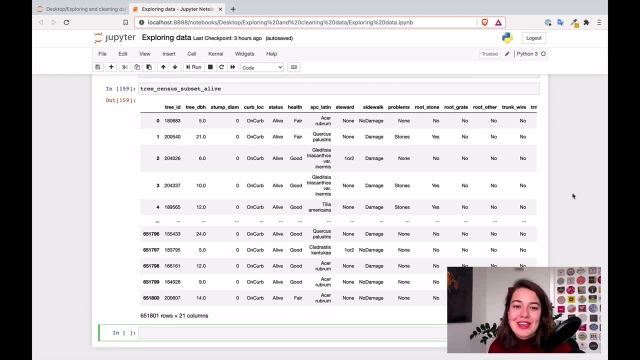 if you came, if you're interested in this video, please subscribe to our channel and hit the bell. if you listened to me the whole way, if you came all the way here- really, congratulations for keeping out with this. um, just wanted to give you, with this video, an explanation of you know, or just a feeling. 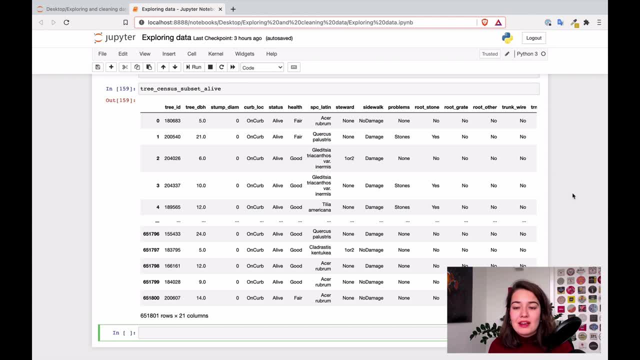 of how a data scientist approaches these things, because, as you see, as you saw, we basically- like you know, i am also seeing this data set for the first time, so there were things that popped up while i'm doing some analysis, and then you know exactly how you are supposed to approach these. 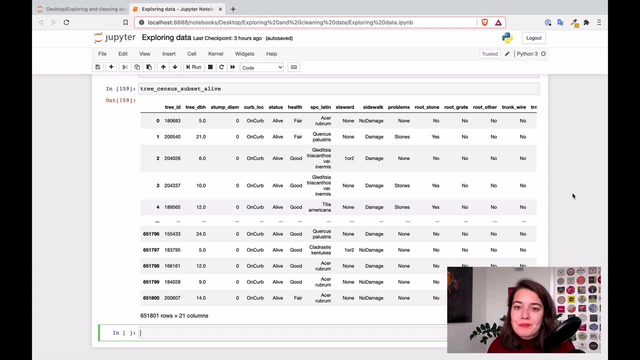 things. you can't know everything from the beginning. you basically create things as you go. you basically, um, come up with solutions as you go. so, uh, let's end this video here. i hope you learned a lot and, yeah, i hope to see you around.